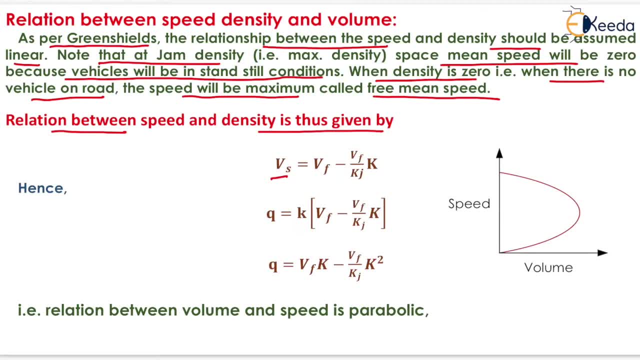 mean speed and Kj is the jam density. Now if we want to determine the traffic volume, then it will be equals to speed into density. So it will be equals to K into Vf minus Vf upon Kj into K. So on solving this we will have Q equals to Vf into K. 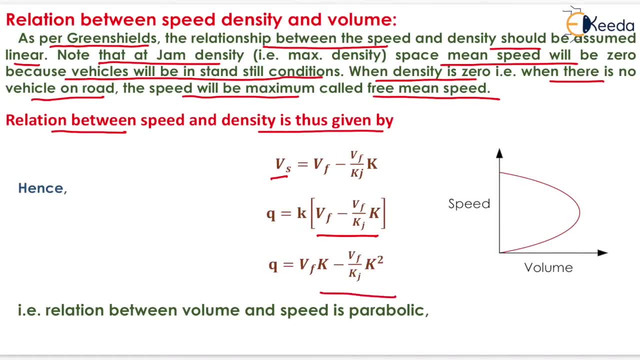 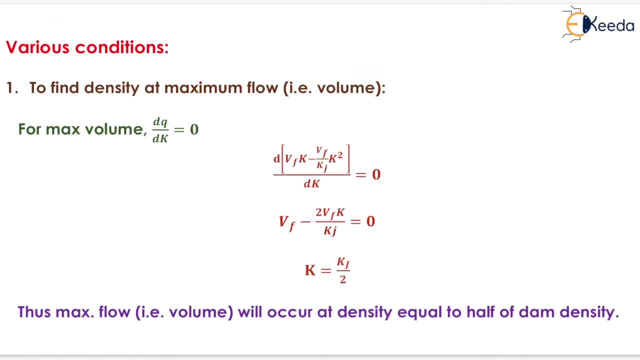 minus Vf upon Kj into K square, that is, the relation between volume and speed is parabolic, which is shown here. Now we have the various conditions. The first one is to find density into density. Now we have the various conditions. The first one is to find density into density. 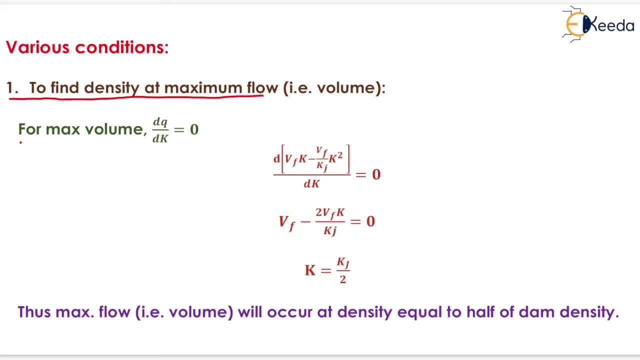 at maximum flow. that is volume. Now for maximum volume, dQ upon dK will be equals to zero. So, on solving this, we will have Vf minus 2 Vf. K upon Kj equals to zero. from this, K will be equals to: 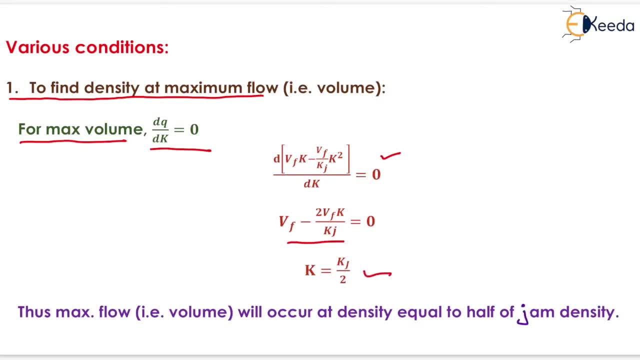 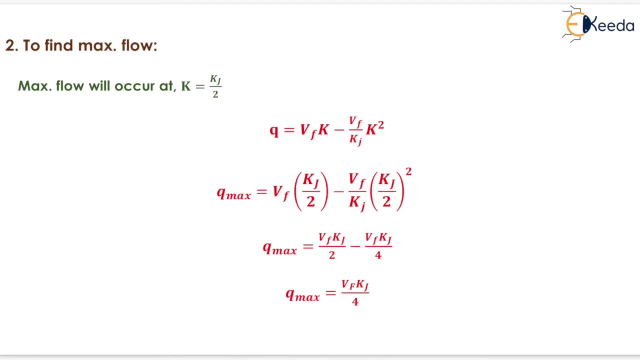 Kj by 2.. Thus maximum flow, that is volume, will occur at density equals to half of jam density. Now the next is to find maximum flow at. maximum flow will occur at K equals to Kj by 2. So Q will be equals to Vf into K minus. 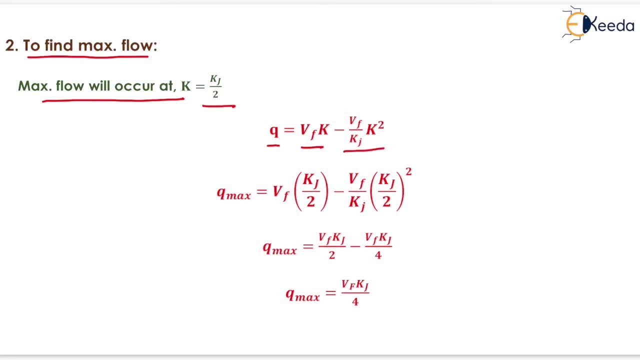 Vf upon Kj into K square. Now for finding the maximum flow, that is, Q max, we have to put the value of K equals to Kj by 2.. On putting the value we will have Q max equals to Vf into Kj. 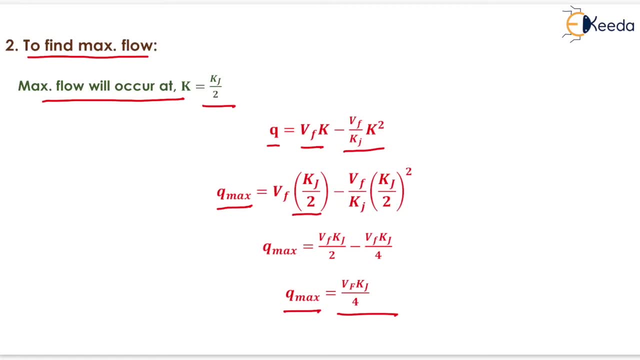 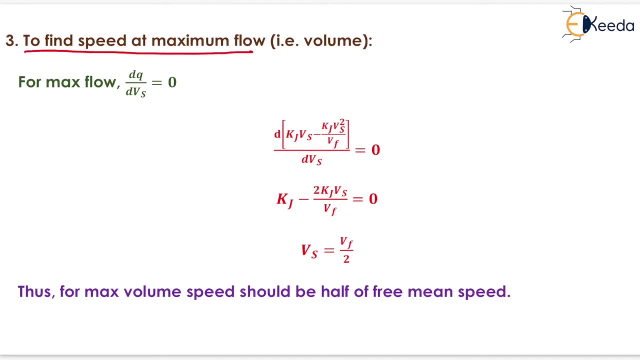 by 4.. That is the 1 by 4, into free mean speed, into jam density. Now the next one is to find: find speed at maximum flow, that is volume. Now, for maximum flow, dq upon dVs equals to 0. On solving this, we will have Vs equals to Vf by 2.. Thus for maximum volume speed, 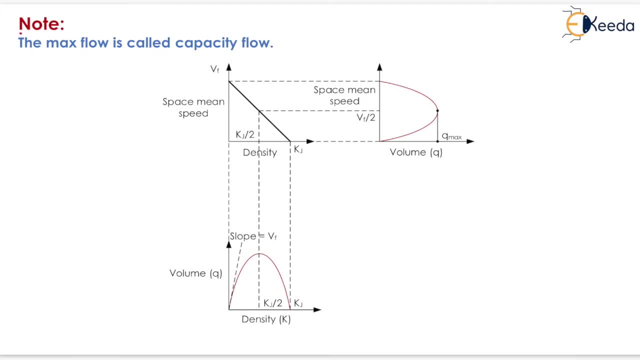 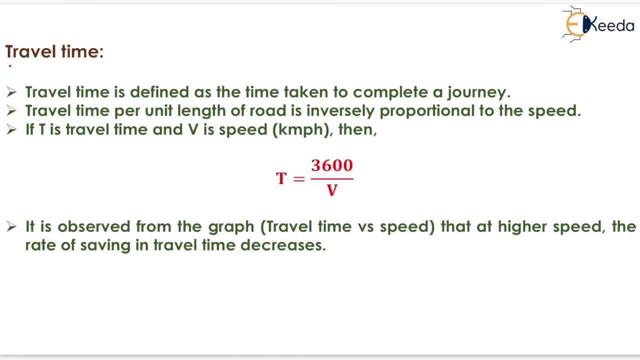 should be half of the free mean speed. Now one note is written here that the maximum flow is called the capacity flow, which is shown here by the curve. Now the next topic is the travel time. Travel time is defined as the time taken to complete a journey: Travel.